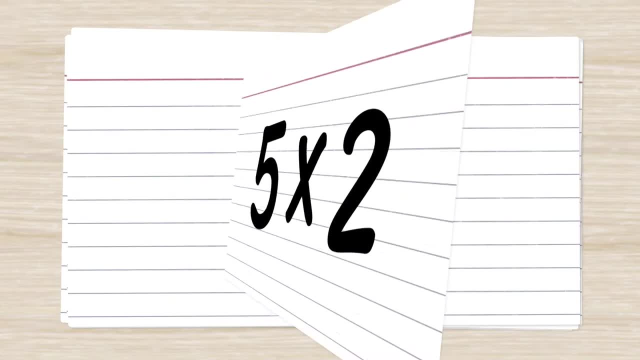 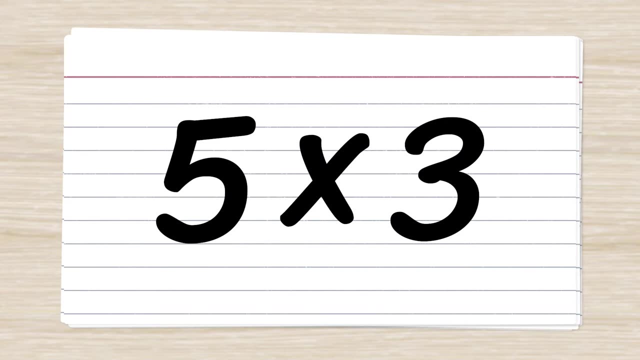 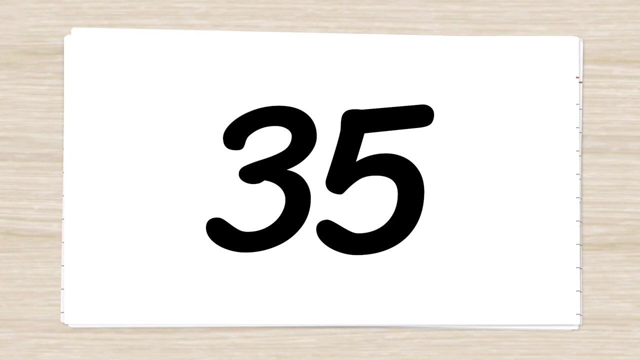 Ten, Five times three. Fifteen Five times four. Twenty Five times five, Twenty-five, 5 times 6, 30, 5 times 7, 35, 5 times 8, 40, 5 times 9, 45, 5 times 10. 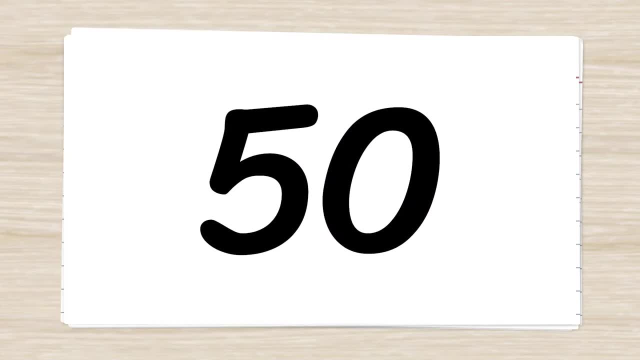 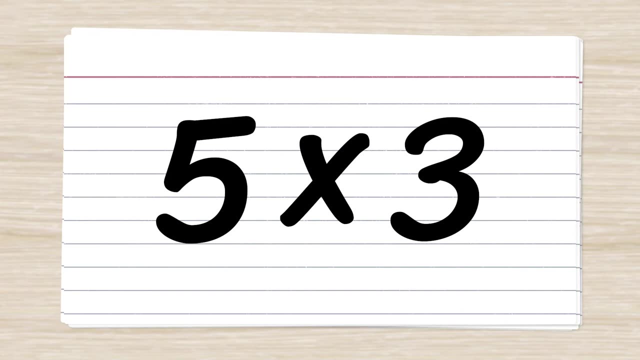 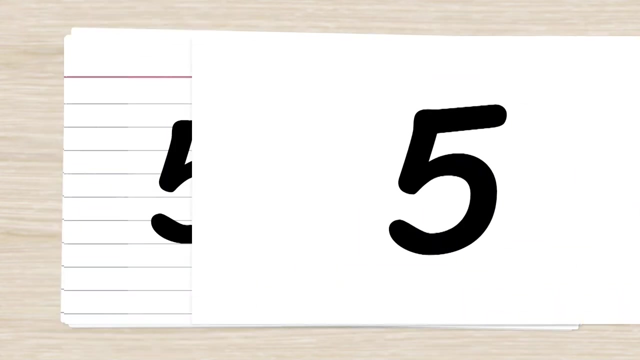 50, 5 times 3, 15, 5 times 4, 20, 21, 5 times 0, 0, 5 times 6, 30, 5 times 1, 5, 5 times 5, 25, 5 times 6. 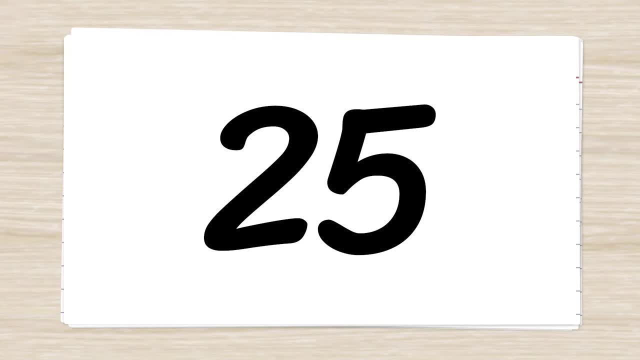 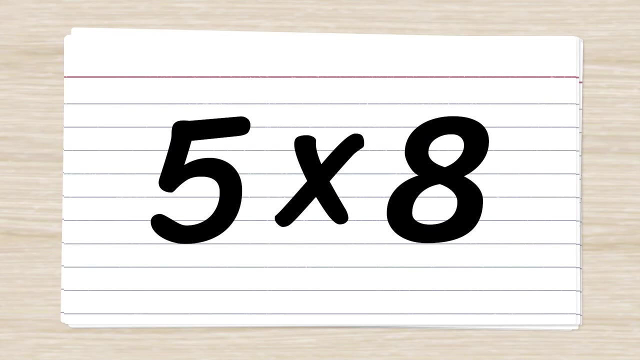 25, 5 times 10, 5 times 10, 50, 50, 5 times 8, 5 times 8, 40, 40, 5 times 9, 5 times 9, 45, 45, 1, 45, 5 × 7.